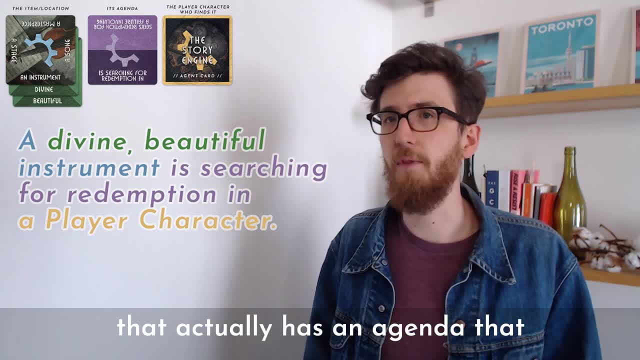 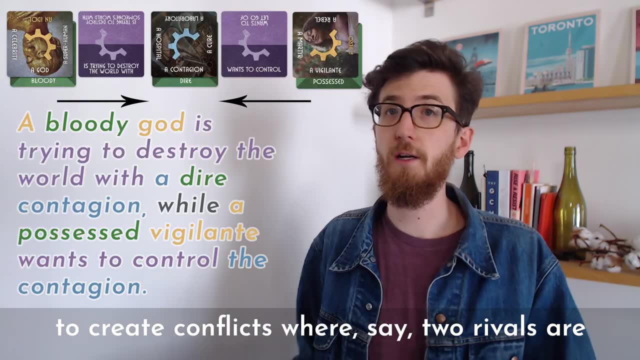 a haunted location or a magic sentient item that actually has an agenda that it's going to imprint on whatever player stumbles upon it. You can also set up symmetrical structures to create conflicts where, say, two rivals are opposing one another and they want the same thing. 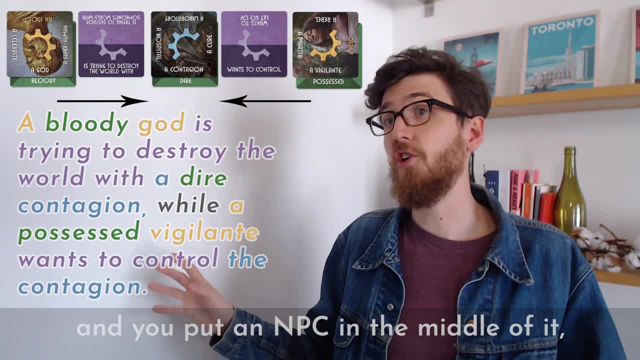 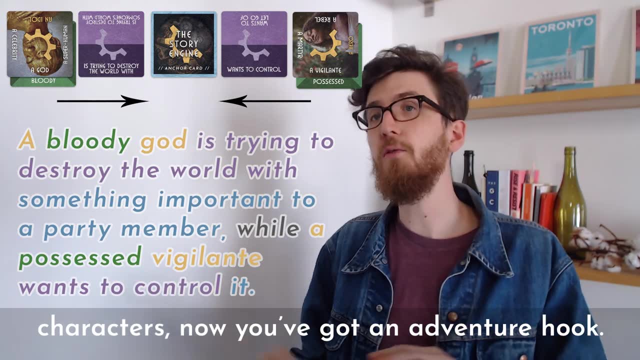 but for different reasons. And if you take this exact same structure and you put an NPC in the middle of it, someone that the players care about, or an item that's important to one of the characters, now you've got an adventure hook. Now you've got a reason for them to be involved in. 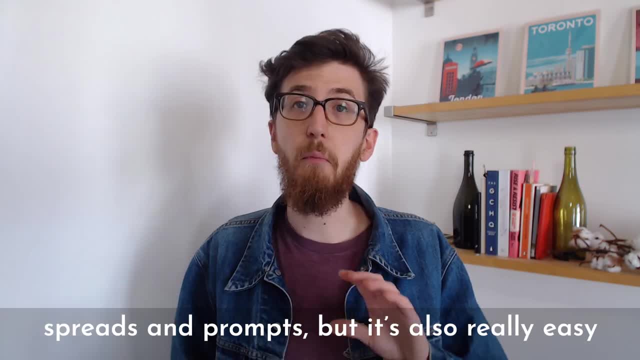 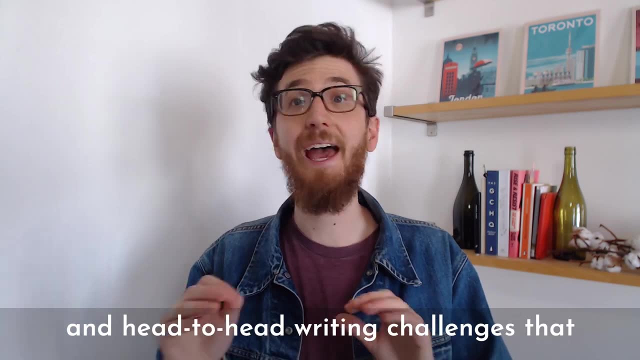 a conflict. The deck does come with all of my favorite spreads and prompts, but it's also really easy to develop your own systems organically. I'm even developing collaboration focused prompts and like head-to-head writing challenges that you can write with your friends. 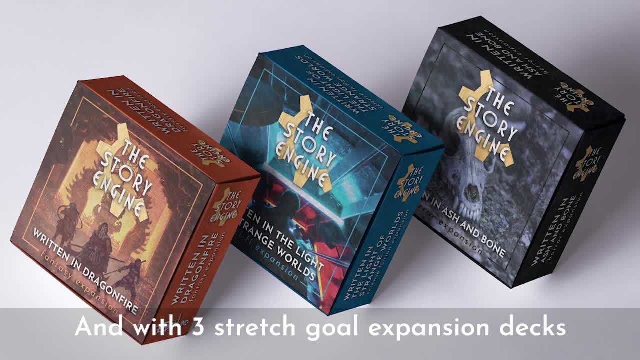 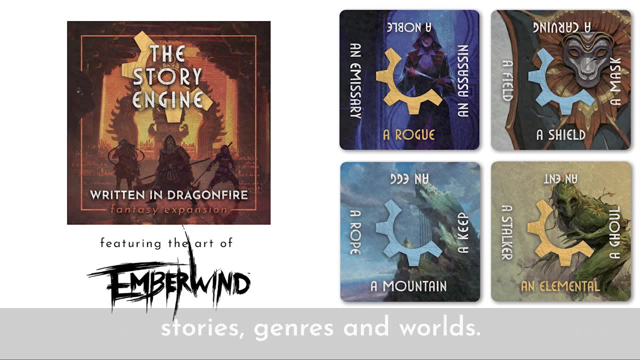 or create stories together in a multiplayer mode And with three stretch goal expansion decks focused on fantasy, science fiction and horror storytelling, you'll be able to explore even more stories, genres and worlds. I have been planning this deck for a long time now. It brings together all the lessons I've learned about storytelling. 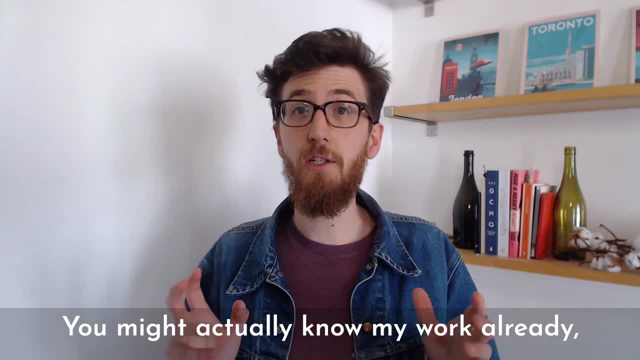 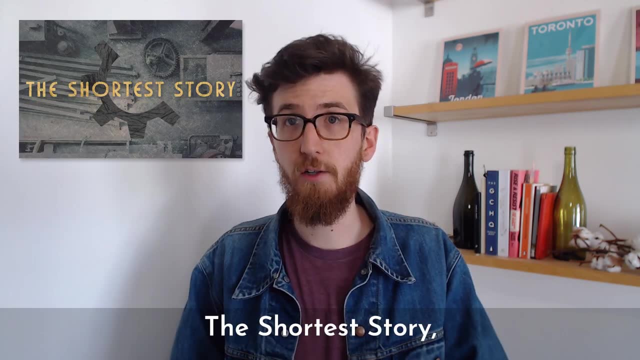 from the past 10 years working as a writer. You might actually know my work already, whether it's from my award-winning webcomic Rock Paper Cynic, or my weekly postcard fiction project, The Shortest Story, one of the tabletop games or video games I've written for, or one of the 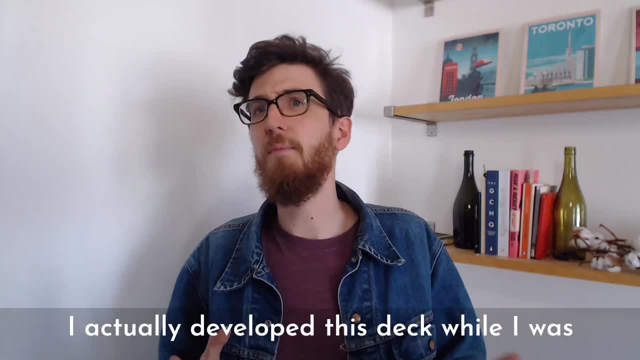 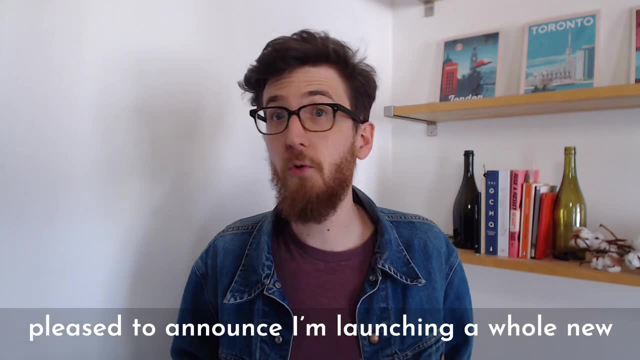 Kickstarter's that I've already run and delivered. I actually developed this deck while I was writing a book of one-page postcard stories for my website, shorteststorycom, and I'm very pleased to announce I'm launching a whole new collection of my microfiction. It's going to contain 90 of my 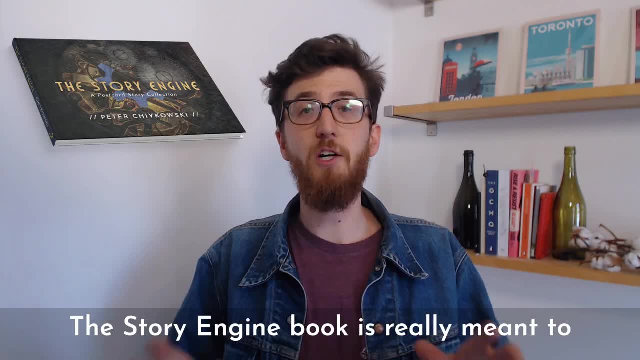 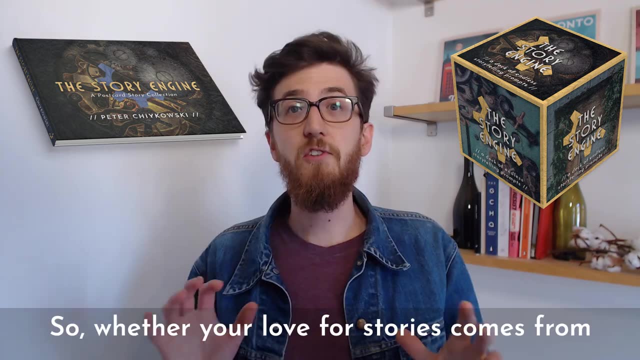 best stories, ones that I wrote while developing the deck. The story engine book is really meant to showcase the thought process that went into developing the deck and also the possibilities that the deck has. So, whether your love for stories comes from reading or writing or gaming, 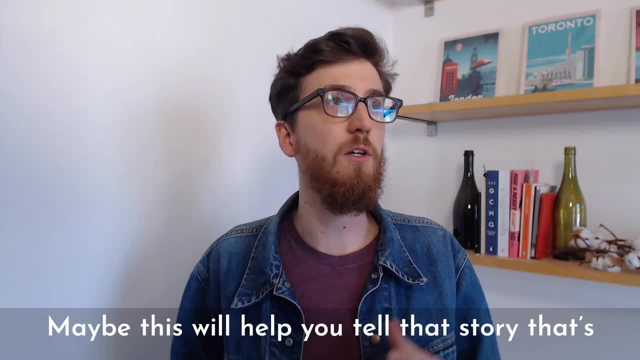 or role-playing. I really think there's something here for you to get excited about. Maybe this will help you tell that story that's been locked up in your head for all these years. or maybe you're already telling stories and this will help you take that to the next level. I'd love for you to